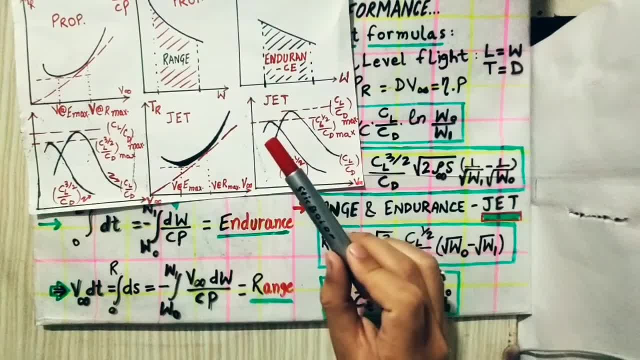 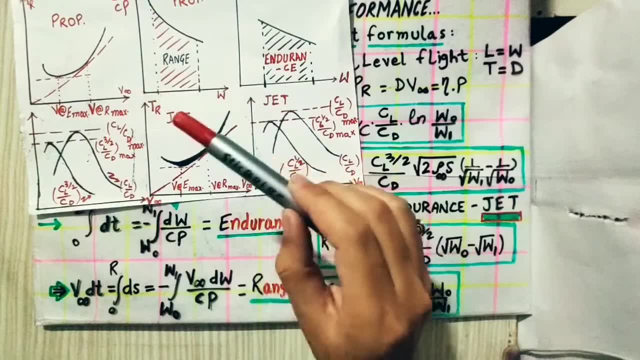 propeller driven aircraft to make its range maximum or endurance maximum. We want to fly at that velocity At which it should cover the maximum range or the maximum endurance. over that is, it should cover the maximum distance, or it should fly In the air with maximum time for a given tank of fuel. Okay, Similarly, we have done this for jet aircraft. 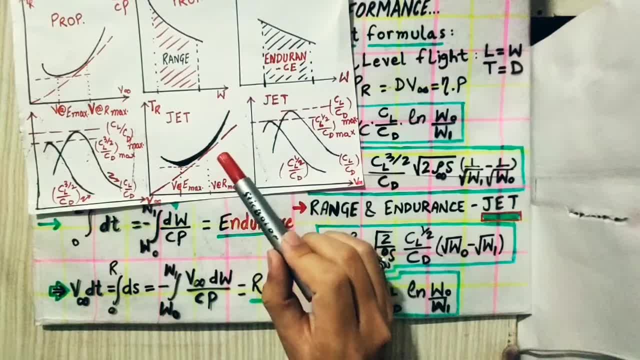 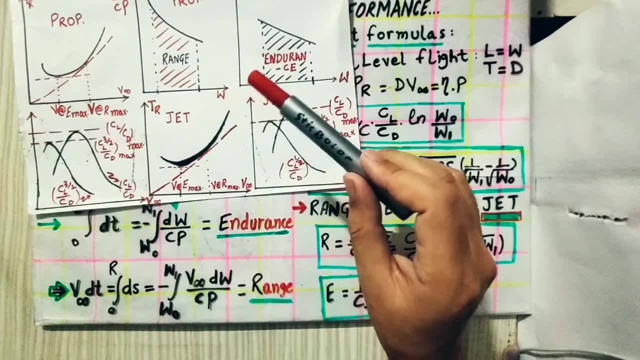 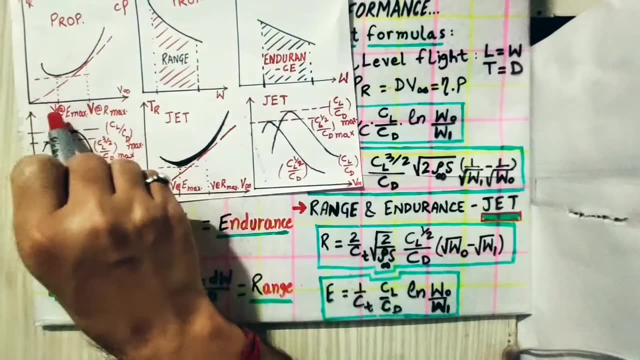 we are relating the velocities, or Getting to know about the velocities for which a jet engine aircraft will be flying at that velocity at which its range will be maximum, Or it will be flying With that much velocity at which endurance will be maximum. So from this graph we have power required. variation like this which shows that power required minimum is this point and velocity at this point. 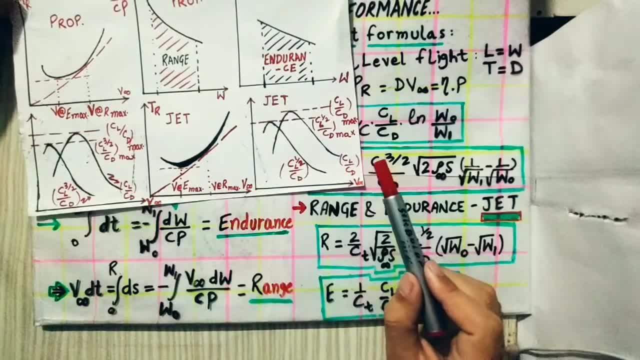 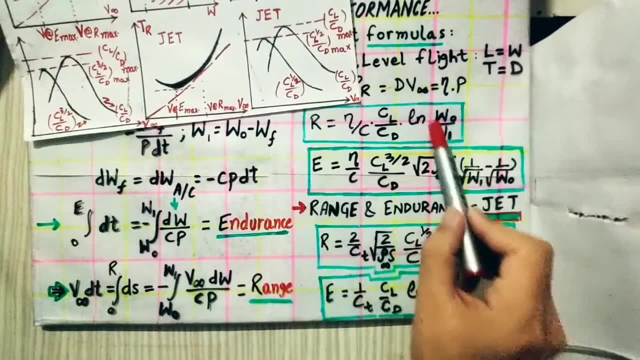 Is the velocity which we get at endurance maximum, that is, we know, the upward power. Endurance is this. So this is the endurance and this is the range for a propeller driven aircraft. now, if we, in 1, 2, fly our aircraft with the rate of has to fly at a certain velocity so that it should cover this. 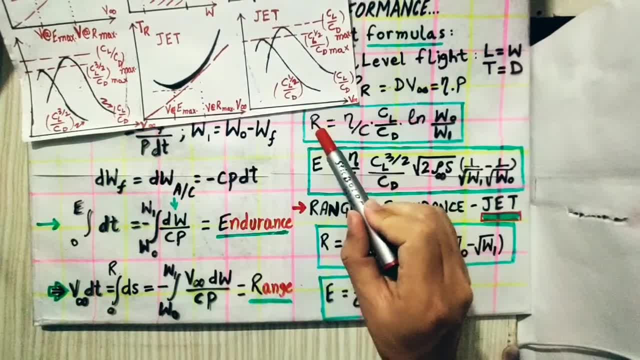 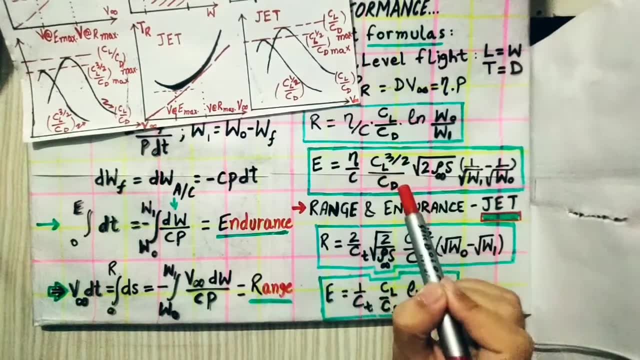 Much range or say it should cover the maximum range and maximum endurance. When the range will be maximum, which is Cl by CD, This should be maximum and for endurance to be maximum, Cl by CD, which cl raised to power 3 by 2 divided by CD. This 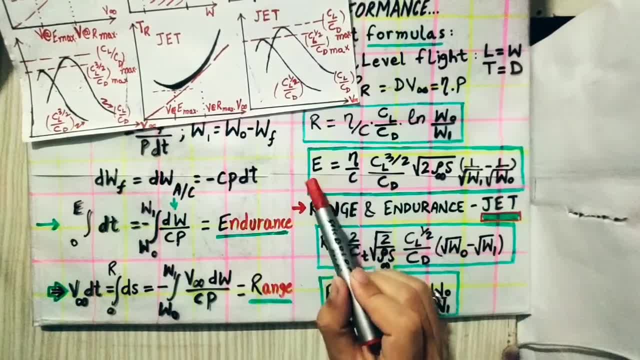 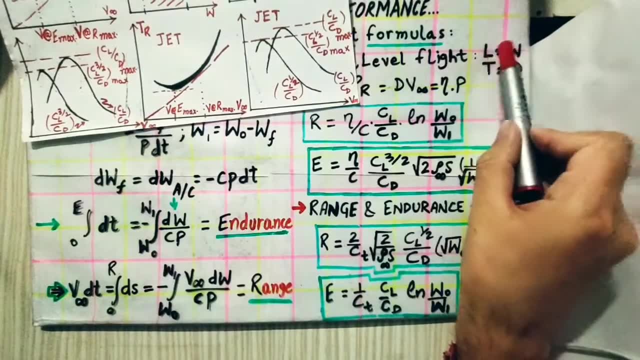 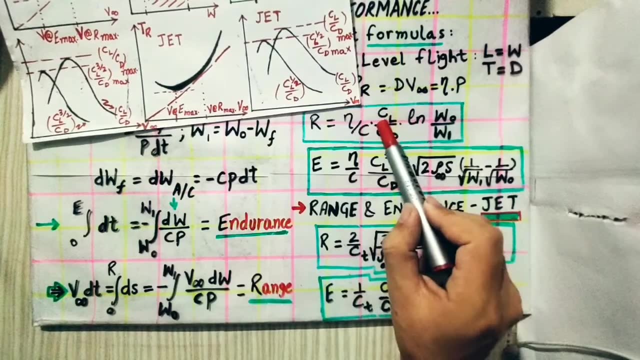 aerodynamic ratios should be maximum, for range and endurance to be maximum respectively, and while it does not know anything about the aerodynamic derivatives or say aerodynamic coefficients, actually, and we know lift equal to weight and from this we can calculate the velocity, knowing about the CL. okay, from that we can compute the CL CD ratio and upon knowing that we can, 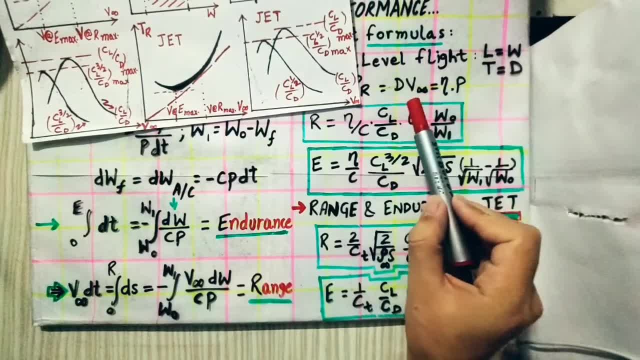 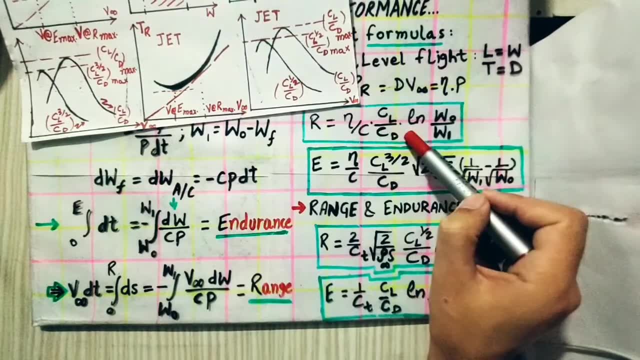 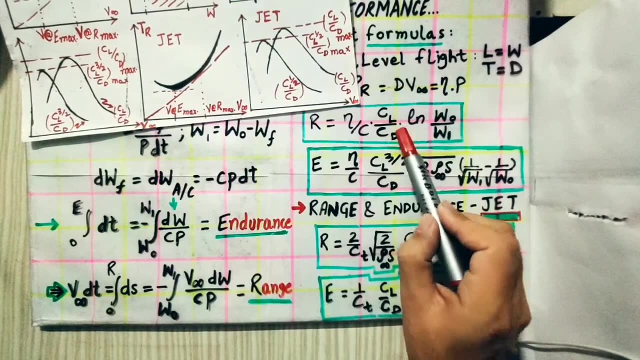 plot the variation of CL CD with respect to velocity and from there we will see that corresponding velocity at which the aircraft will be flying will be with respect to CLF CD max for range maximum. actually, we will be learning about the velocity at which CLF CD is maximum, for which we know the range will be maximum. 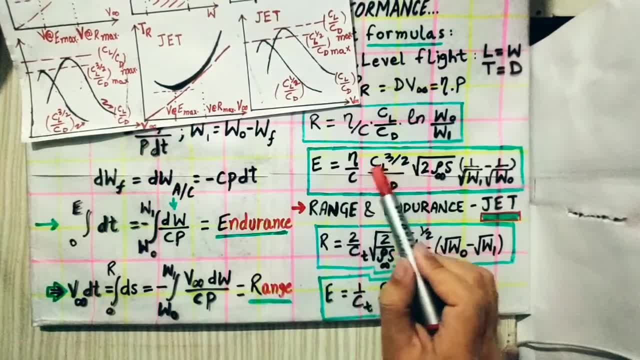 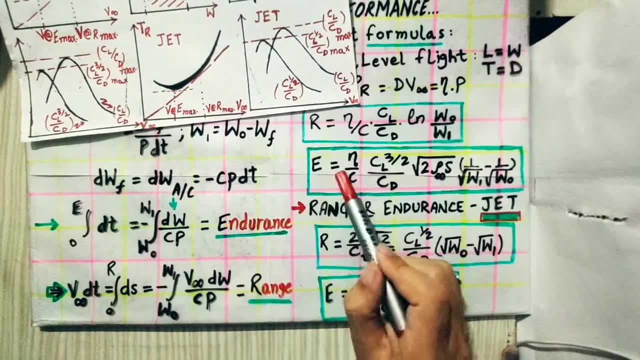 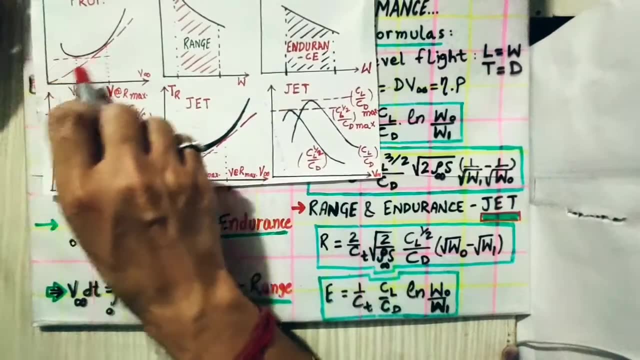 similarly we will see, see less, about three by two will bealey CL velocity. we will compute and from there we get to know about the endurance, at which velocity it gives us one up, a two, two by Cd max. that velocity we will see endurance will be maximum. so from this graph we have power required minimum. 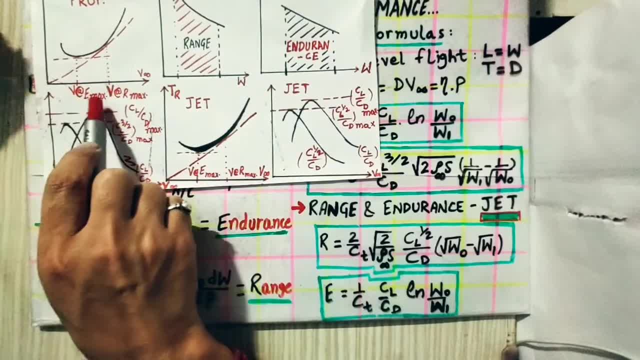 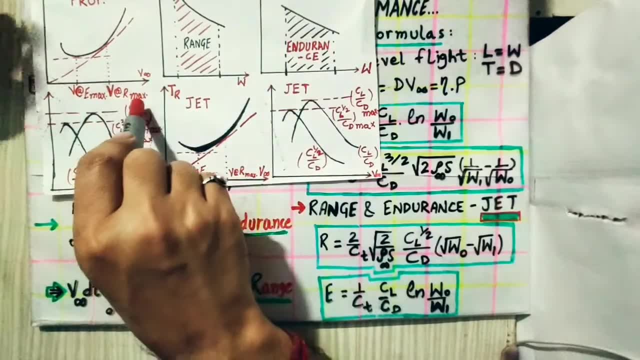 over here. vélocity correspondence velocity would represent therell στο into. this is also the velocity at which the endurance is maximum. and when the tangent is drawn at any point on the curve, the minimum tangent on this curve gives us the velocity at which the range is maximum for a propeller driven aircraft. and from the formula of range 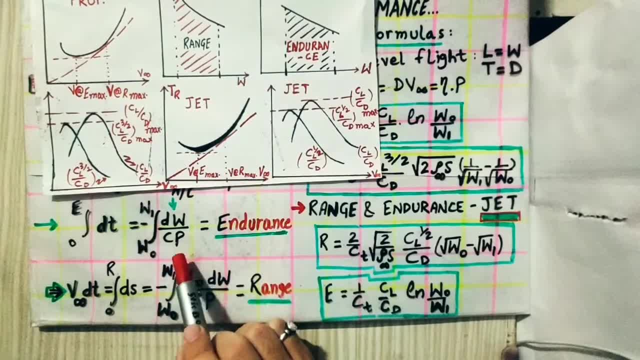 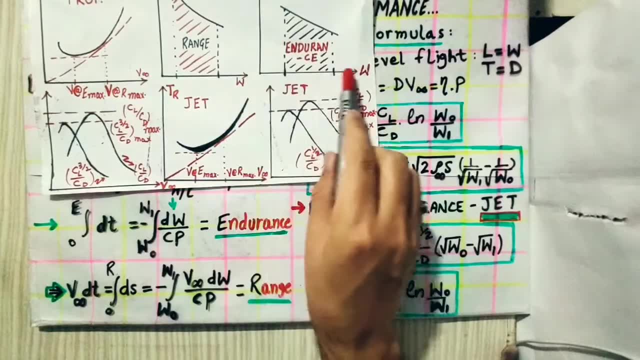 and endurance over here. we know that endurance is dw by cp. okay, so for initial weight w naught and final weight w1: initial w naught and final w1. and we know the aircraft weight changes over a period of time. it decreases actually, which is why it is decreasing, and when this instantaneous. 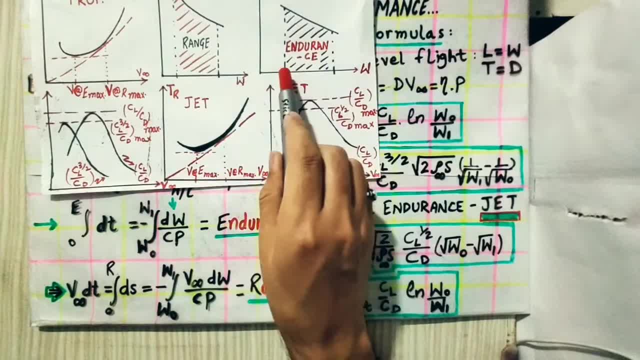 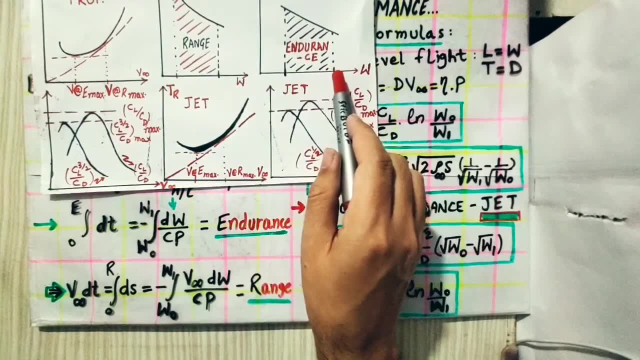 weight multiplied by 1, by cp, will give us the endurance for a change over a period of time. actually, uh, it will be for initial and final weight of the aircraft when the whole weight of the fuel get consumed. okay, so the endurance will be then the area under this curve, because 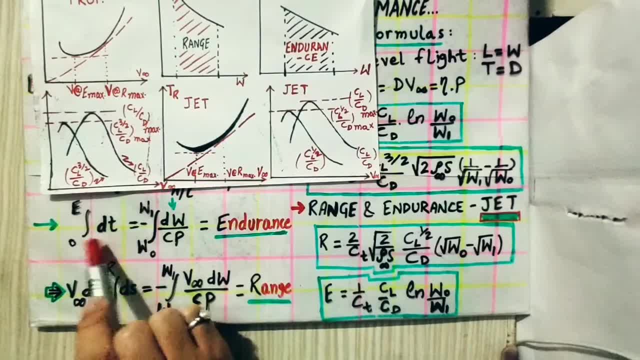 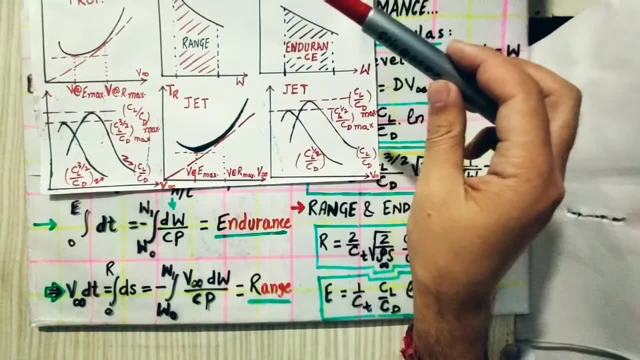 we know from this, integral dt is a time interval. okay, upon integrating the time interval and upon integrating this dw by cp, we will get the endurance or the time period. maximum time it will fly in the air, okay. similarly, upon multiplying with infinity, we will get time into velocity as 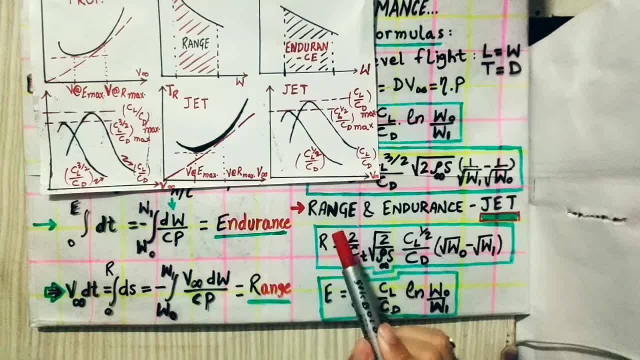 distance, which tells us about the range aircraft will cover, and uh, with respect to the earth surface while flying in the air. okay, so uh, from here we see that v, infinity by cp multiplied by dw will give us this range. so, infinity by cp multiplied by dw, when integrated over a range, 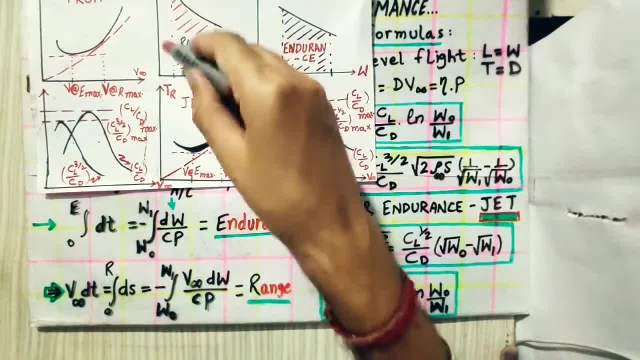 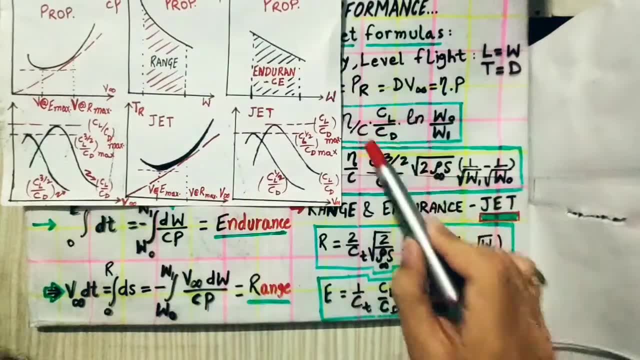 of w naught to w1, similar to this graph, we get the range for this shaded area. so now, moving on to this graph that tells us about the aerodynamic ratios, like here, we look at that cl by cd ratio. we covered that uh, for cl by cd ratio, or cl is about three by two by cd. 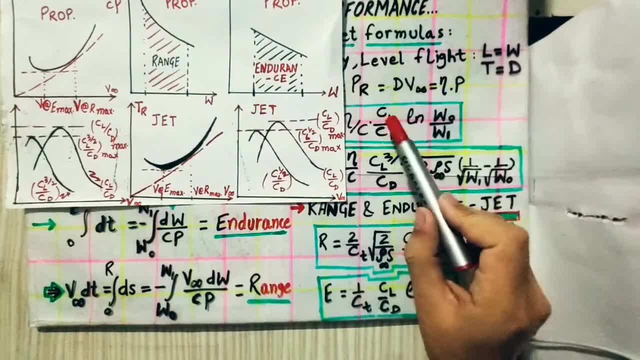 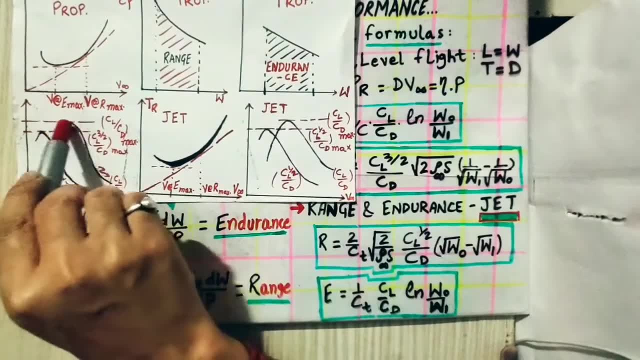 ratio for propeller engine we are talking about and their variation with velocity. we are exploring over here that, uh, cl by cd variation is like this: and cl is about three by two by cd. is this and this is the maximum point at which cl by cd is max? okay, c? l by cd. is this curve and for this? 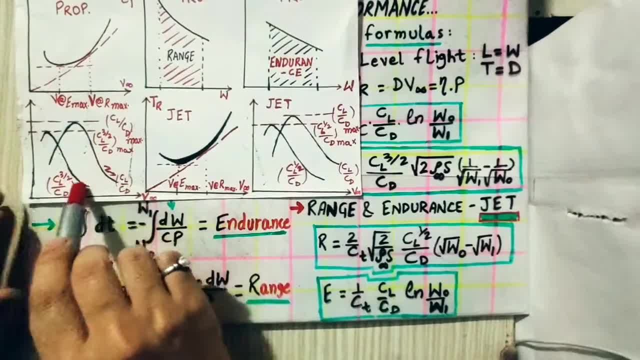 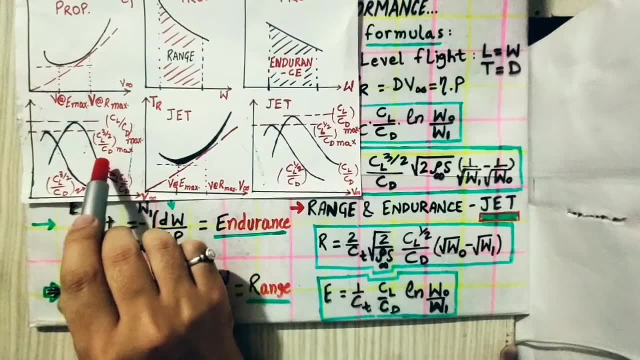 curve: cl by cd is max at this point and for cl is about three by two. by cd it is this, and here it is less than this cl by cd, because as cl increases, cd also increases, because we know cd is a function of cl as well, because cd is equal to cd naught plus cdi, where cdi is equal to. 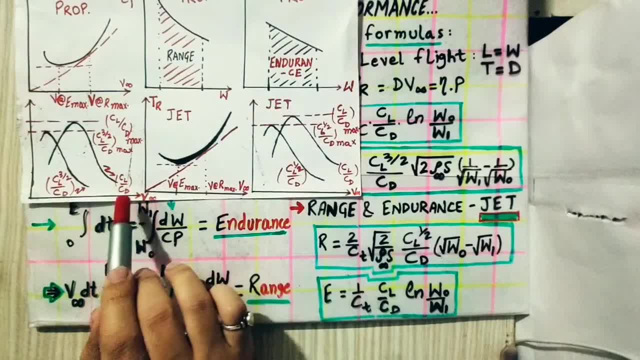 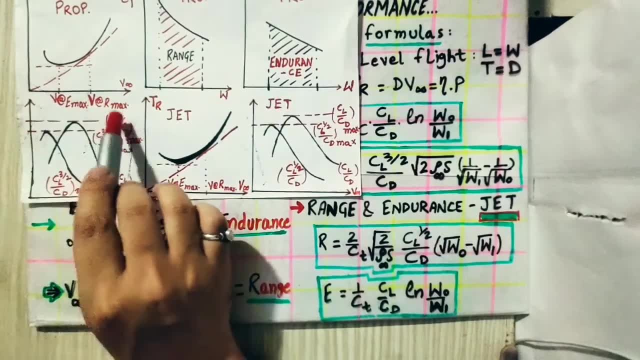 kcl square. okay, so as cl increases, we know velocity decreases. okay, so as velocity increases, increasing over here. therefore, cl is decreasing. okay, so cl upon, when it is cl is decreasing, the numerator will have a value of 0.5 or 0.3, something like that. so, based on that, this: 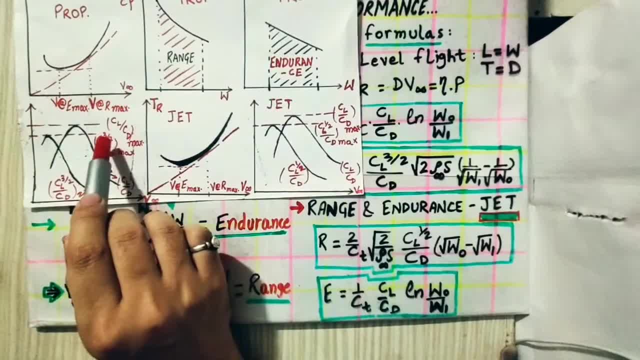 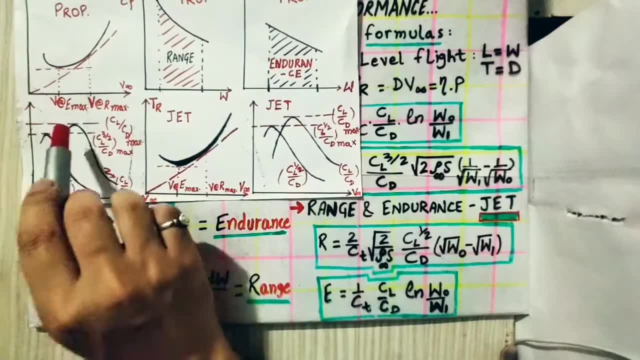 will be having higher values. that's why it is going above this graph. and when, let's say, 0.5 is here and 0.5 raised power, 1.5 will be even lower value. okay, that's why we have this graph, this curve and velocity corresponding to this cl by cd max is the velocity at which the range will. 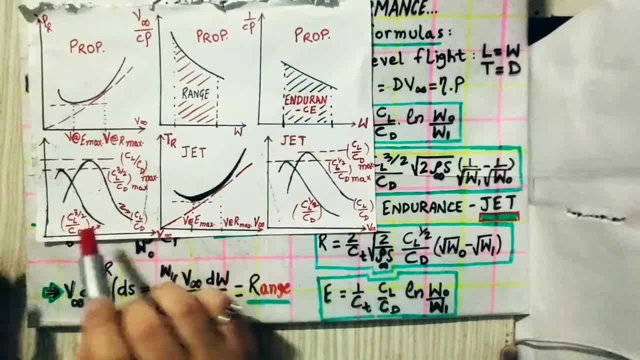 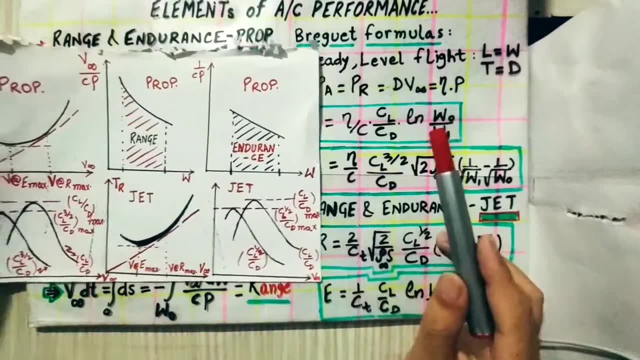 be maximum for cl by cd max. okay, and for this we have cl raised about 3 by 2 by cd max, that is velocity at which this endurance will be maximum for the propeller driven aircraft, which is actually operated by a reciprocating engine. and now, moving on to the jet aircraft, we 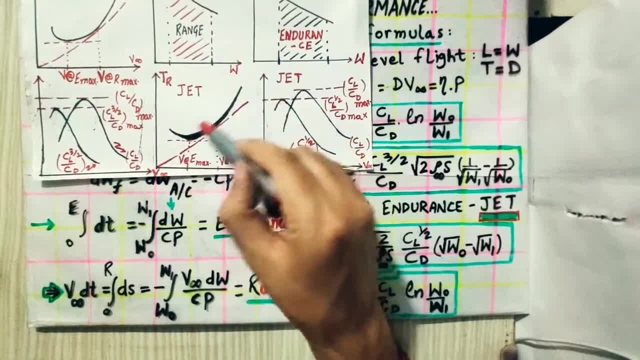 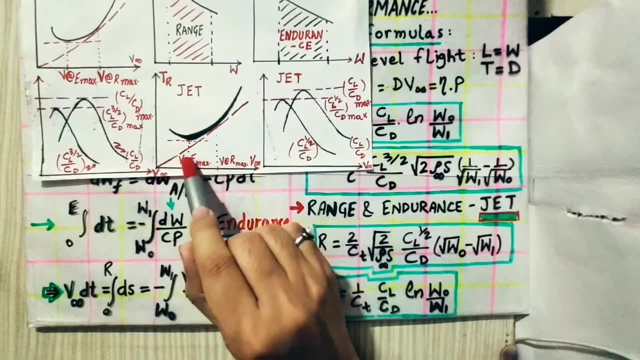 see that thrust required that is equal to drag, which is directly proportional to v square. we know this by heart. and this is the quadratic curvature, we will say that, uh here, if we will see that required is minimum at this point and velocity corresponding to this is the velocity at which. 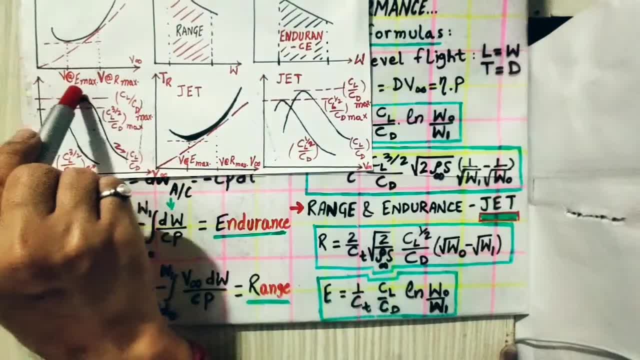 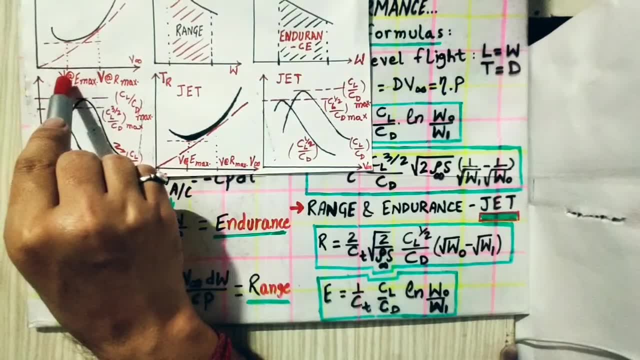 endurance is maximum, just like propeller power required minimum at which the velocity is maximum for a velocity, power required is minimum for an aircraft at that velocity and when the aircraft fly at power required minimum it will cover it will stay in the air for maximum time, which is why 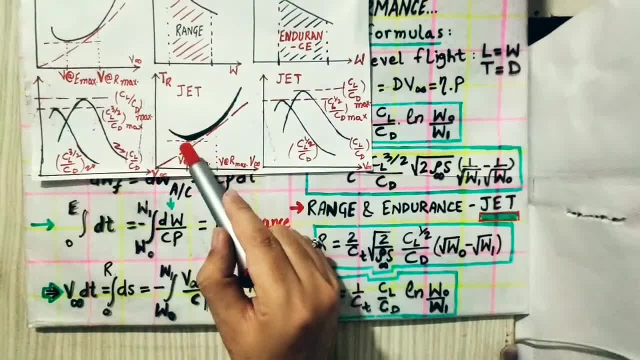 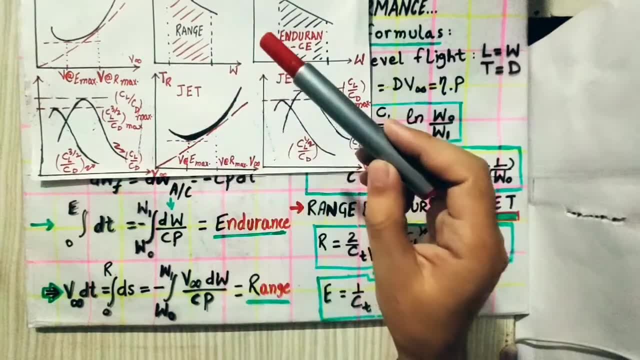 we are having the velocity corresponding to the maximum endurance. similarly over here. if the aircraft flies at the minimum thrust required here and that will be the velocity at which the aircraft flying to be in the air for the maximum time, and that velocity will be correspond will correspond. 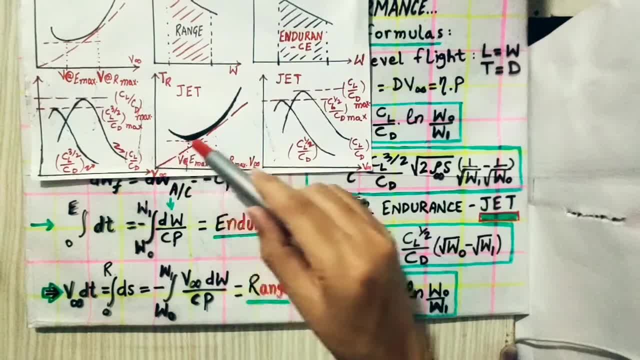 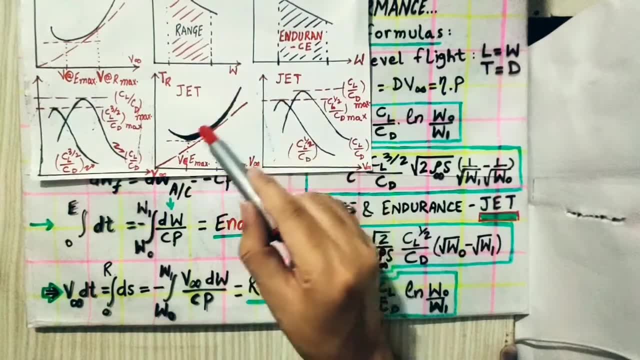 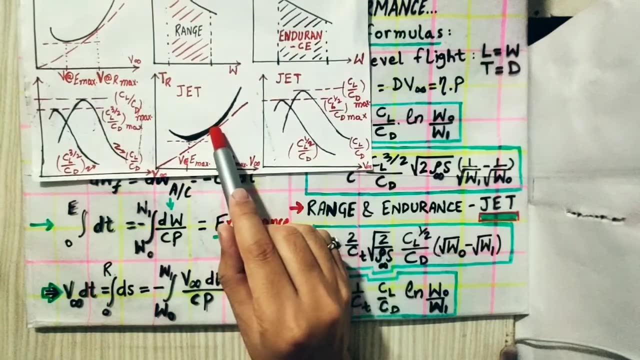 to the maximum endurance, okay, which is ultimately the such required minimum point. and for here endurance, maximum velocity is the power required minimum point. and similarly over here, for the tangent drawn over this curve at any point is minimum at this point. okay, so at this point here we saw that range is maximum for this point because, uh, at this range maximum we see cl is. 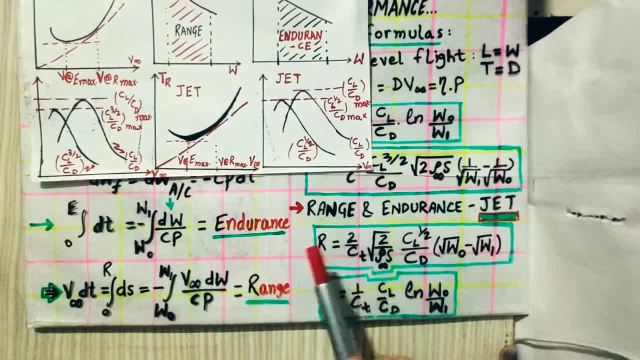 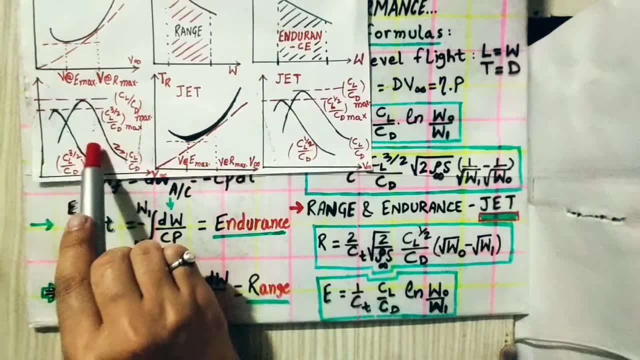 about one by two by cd max and the velocity corresponding to this cl. one by two by cd max, is when the range will be maximum and it is this velocity okay, and similar to this, aerodynamic variation with velocity okay, aerodynamic variation or aerodynamic ratios with velocity for jet engine.